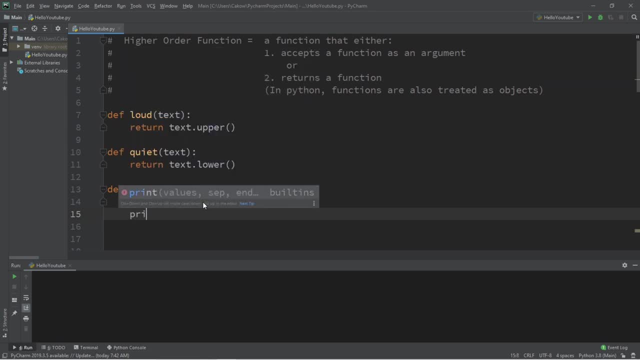 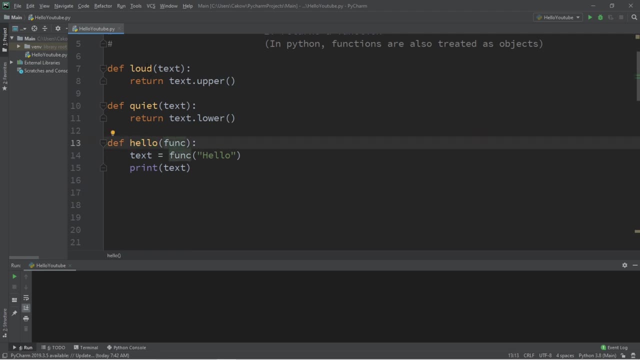 I will pass in just the word hello, That's capitalized At the end. I will print whatever text that we have In order to call this function of hello. I need to pass in a function as an argument. Do I want to pass in loud or quiet? 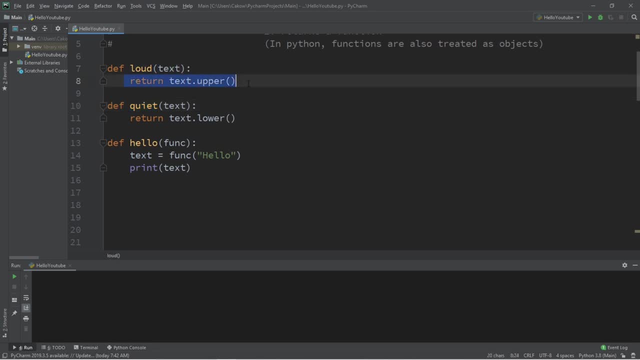 Do I want the loud variety of hello where all of the text will be uppercase, or the quiet variety of hello where all the text will be lowercase? I would like to pass in loud because I want to make my text all uppercase, so I'm typing the name of the higher order function. 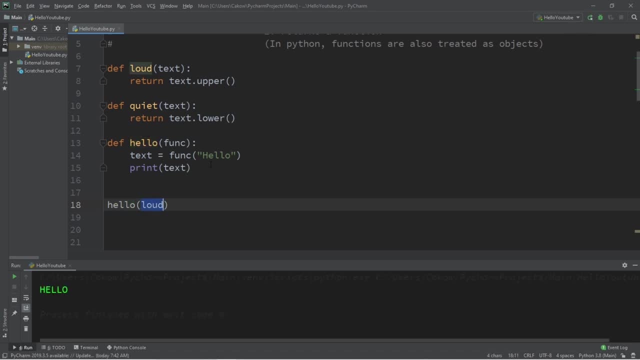 and passing in a function as an argument, and the result is that the word hello will be printed to the console window all uppercase. Now here's a rundown of what just happened. We're calling the hello function and we're passing in loud as an argument. We're naming loud as func while we're 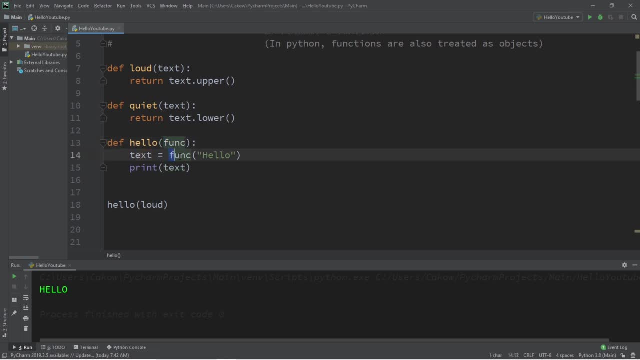 within this hello function, Text equals loud and we're sending a string of text that says hello. We're returning that text all uppercase, assigning it to a variable called text and printing that text to the console window. Now, if I would like to use the quiet variety of hello, 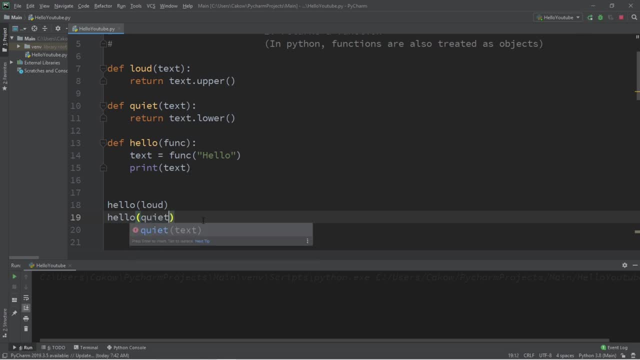 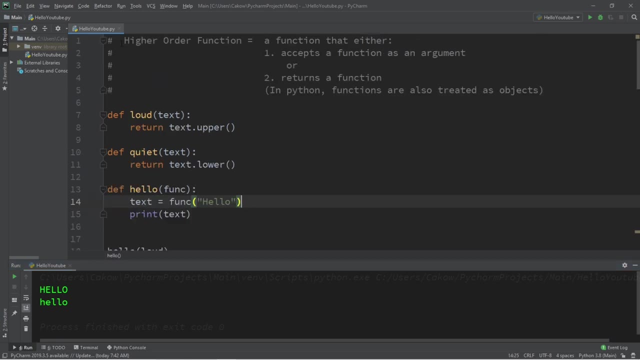 then I'm going to pass in quiet as an argument, So quiet will make all of this text lowercase All right people. so that's example one of a higher order function. A higher order function is a function that accepts a function as an argument. This hello function is an example. 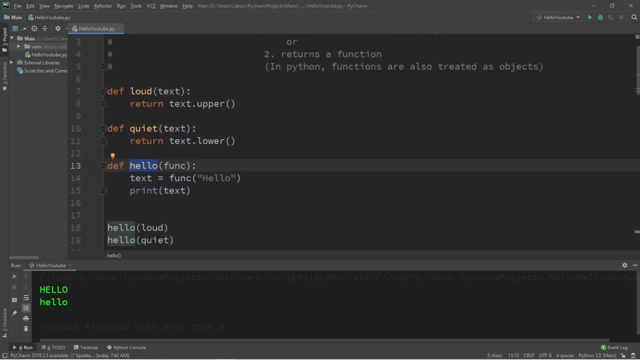 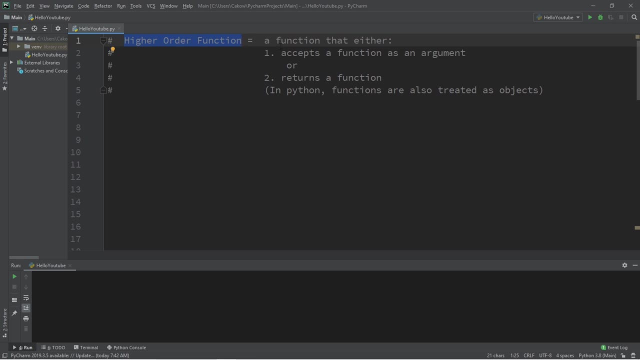 of a higher order function because we're accepting either loud or quiet as arguments. All right, people, let's move on to the second part of this definition for higher order functions. A higher order function is a function that returns a function. I'm going to give a different example. 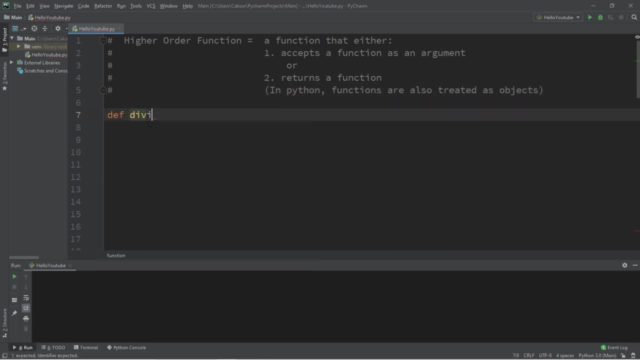 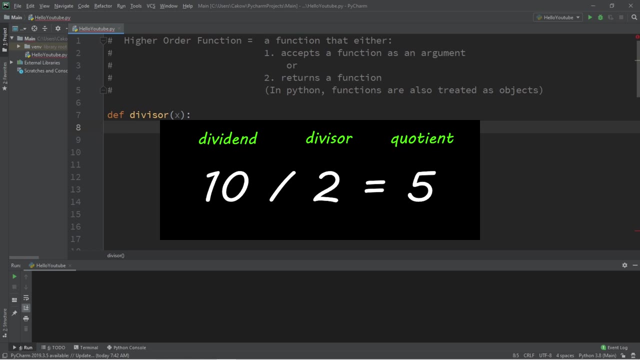 this time. Let's say we have a pair of nested functions. The outer function will be named divisor and we will accept a number as an argument that we will call x. A divisor is a number that is used to divide another number when using division, and inside this function we have an inner function. 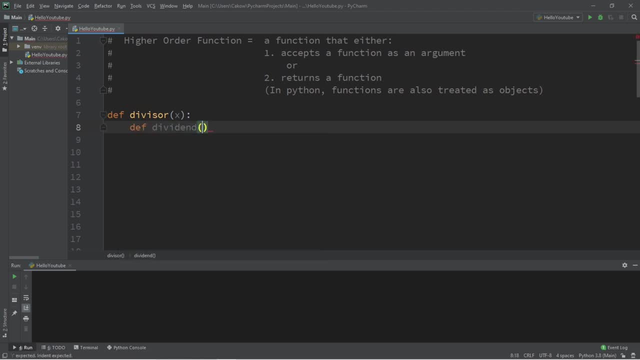 named dividend. Dividend is the number that's going to be divided and we will call the argument that is passed in y. All we'll do is return y divided by x. We're dividing the dividend by the divisor y divided by x, Now within the outer function, but not within the inner function. 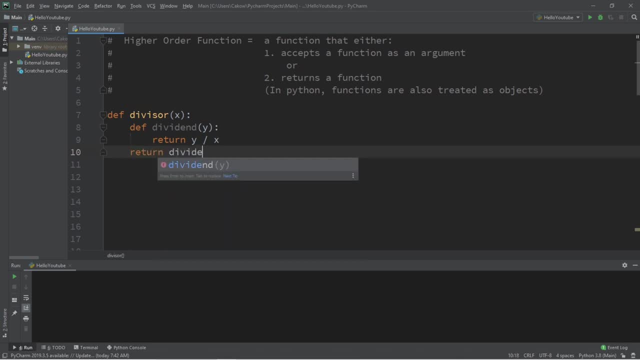 we're going to return our dividend function. So a higher order function is a function that returns a function. Divisor is a higher order function because we're returning dividend. Now if I would like to access this nested dividend function, I first need to call the outside divisor function and pass in a number as an argument to 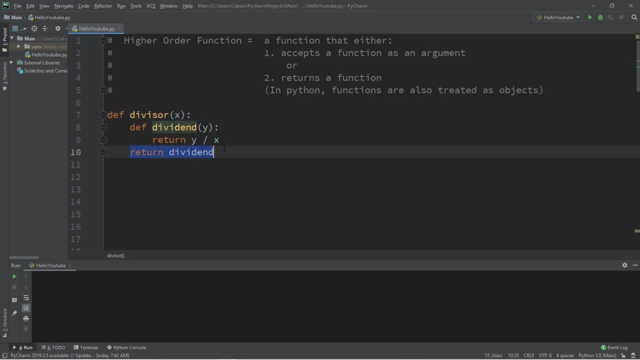 serve as the divisor. The divisor function is going to return my dividend function, which we can then assign to a variable. So the variable I'm going to name divide- Divide equals and I need to call the outside divisor function Divide equals and I need to pass in a number. 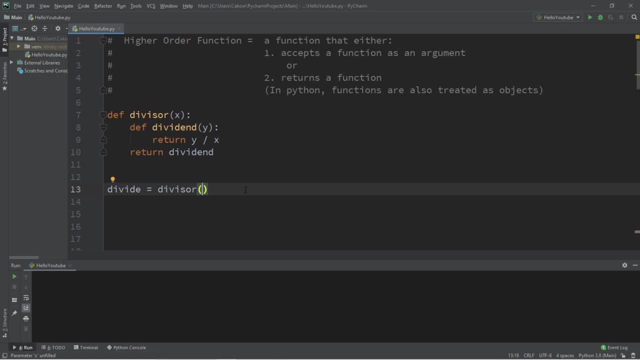 to serve as the divisor function. Divide equals and I need to call divisor and set a divisor. Let's say that I would like to divide all numbers by two, So I will set x to be two. and now for the dividend. I will print, call the divide variable and pass in a number as the dividend, The number that's going. 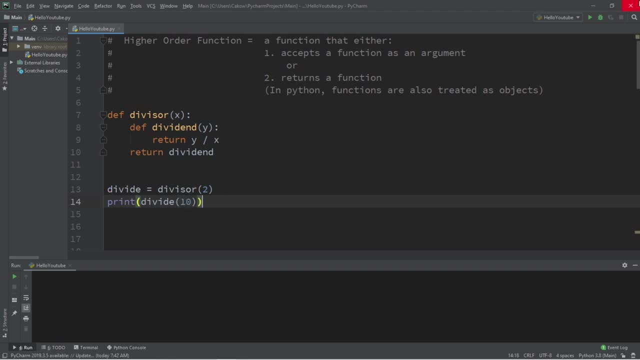 to be divided and let's say I would like to divide 10 by 2 and this will work. As you can see, we have five in the console window, So let me explain what just happened. So our program begins here: Divisor, and we're passing in two. X will be two and it will stay. 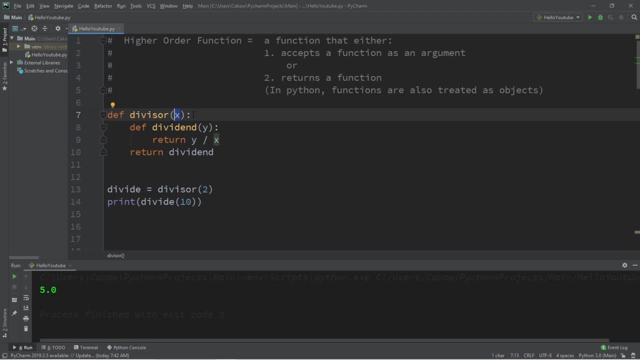 that way until we finish this program or until we reassign x. Now x equals two. We're skipping this function because we did not call it yet. We're returning dividend and assigning it to a variable. and we can call a variable if it has the memory address of a function. 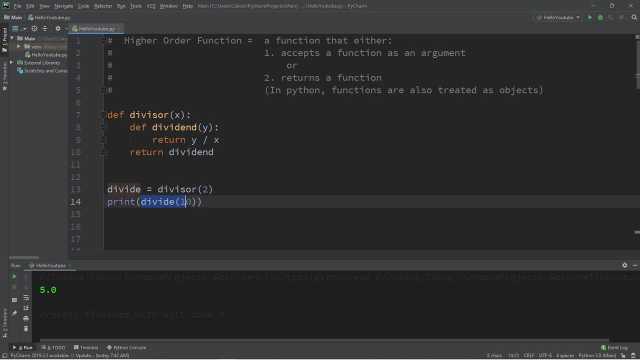 which is what we're doing in this line. Now we're calling dividend and passing in 10.. So y equals 10 and x still equals two. We're returning 10 divided by two and printing it to the console window. Well, everyone. in conclusion, a higher order function is a function that either 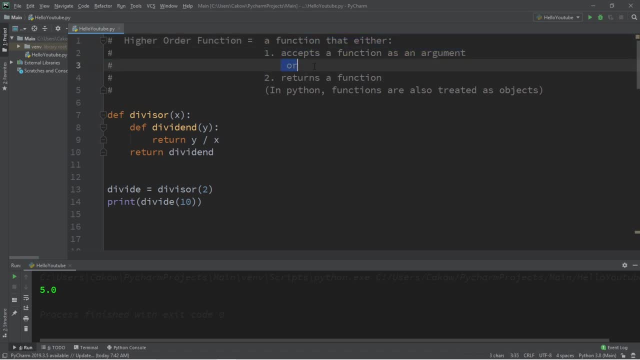 one accepts a function as an argument, or two, they return a function. The format is a little bit strange and we're not quite used to it yet, but in future videos we'll have more practice with higher order functions. If you would like a copy of all this code, I will post all of this. 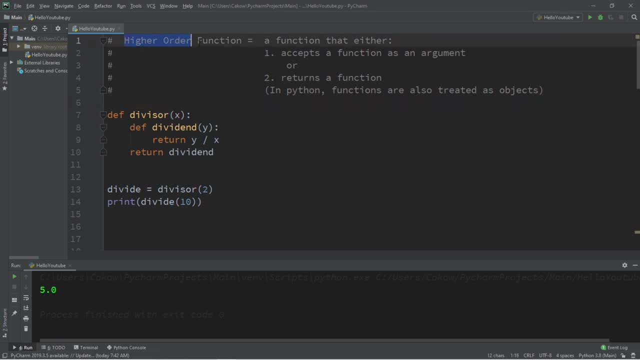 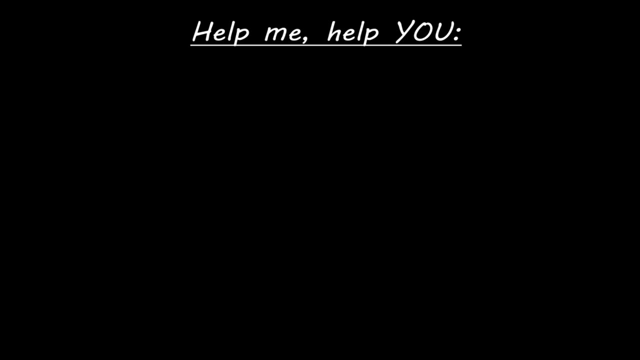 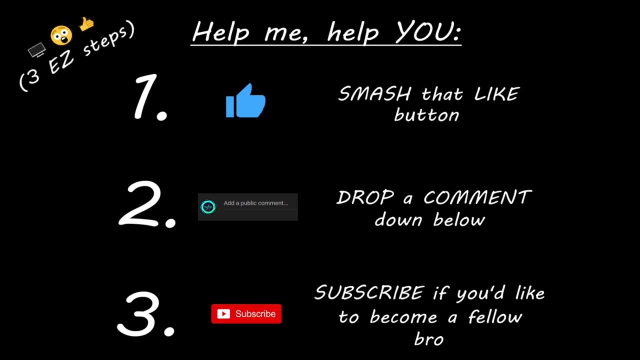 to the comment section down below. Hey you, yeah, I'm talking to you. If you learned something new, then help me. help you in three easy steps by smashing that like button, drop a comment down below and subscribe if you'd like to become a fellow bro.